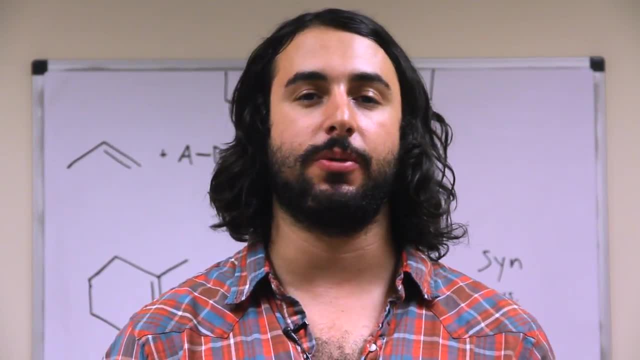 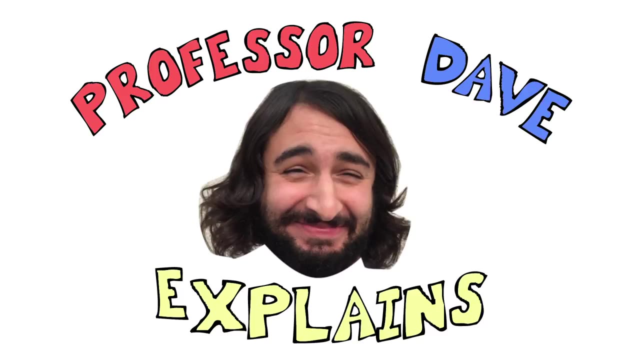 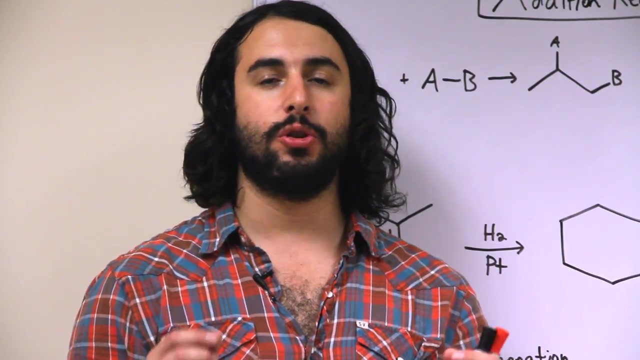 hey guys, professor Dave, here I want to talk to you a little bit about addition reactions. so addition reactions are a little bit like the opposite of elimination reactions, whereas in elimination reactions two groups are removed from adjacent carbons and replaced by a pi bond. here we can see. 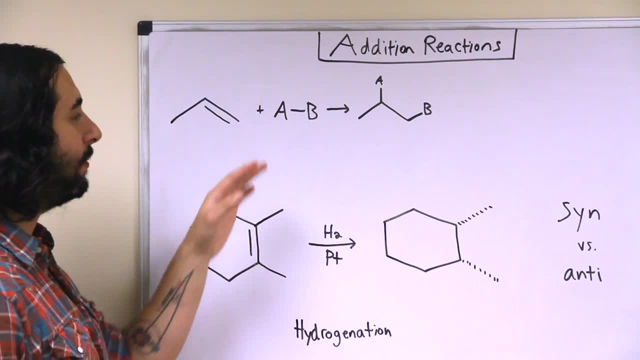 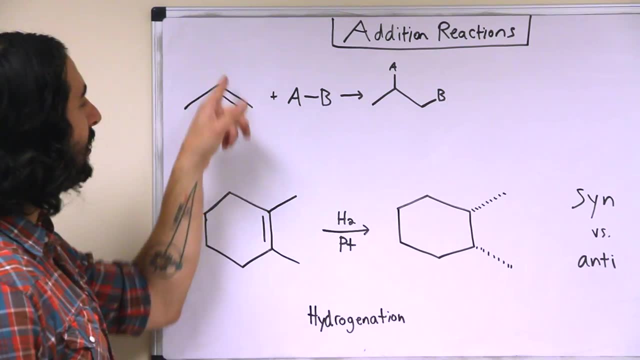 that an addition reaction involves two groups being added to adjacent carbons with a pi bond, and that pi bond is now gone and now those sp2 carbons have become sp3 carbons. so it's a little bit like the opposite of elimination. so 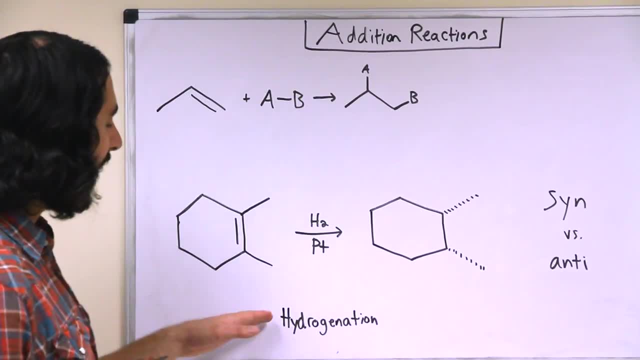 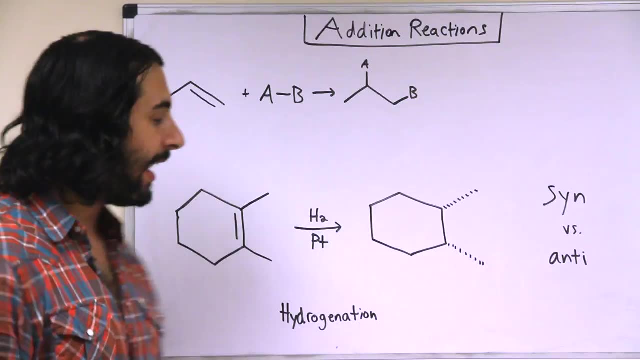 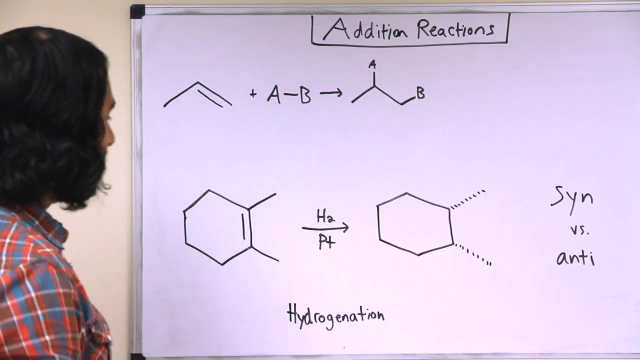 let's take a take a look at one. to start with, we're gonna look at hydrogenation. so hydrogenation is telling us that it's hydrogen atoms that are being added to these carbons, and typically this is done with some kind of transition metal catalyst, a lot of times platinum. so what's happening here is two hydrogen. 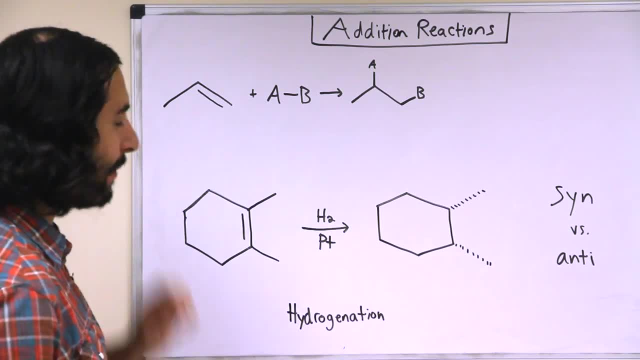 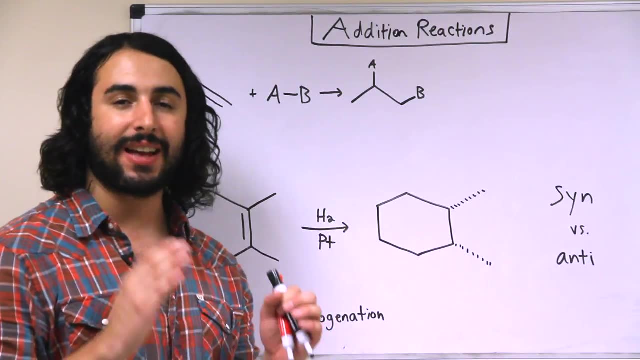 atoms are being added to these carbons and the hydrogen atoms are being added to the two carbons participating in the double bond and in this case, because this is heterogeneous catalysis, this means that the catalyst is in a different phase than the substrate, so it's like a surface that the substrate will. 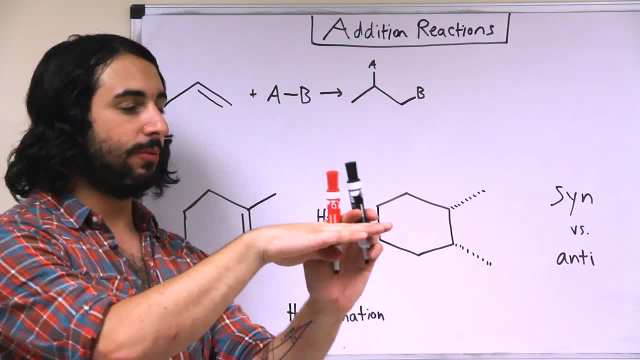 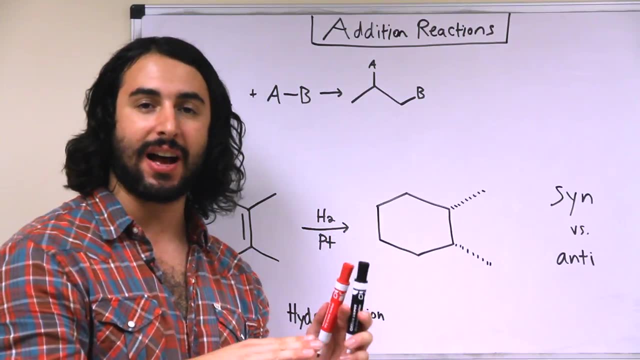 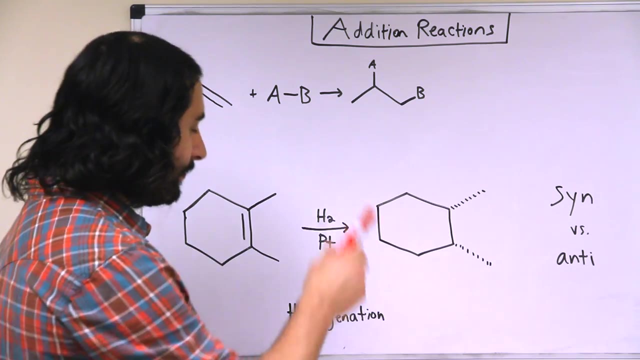 have to approach, and then hydrogen atoms, which are sort of sticking out of the top of the the material, are going to be added, therefore, to the substrate on the same side. so the first thing we have to understand about addition reactions is that they can be stereo specific. so in this case we have to learn the terms syn. 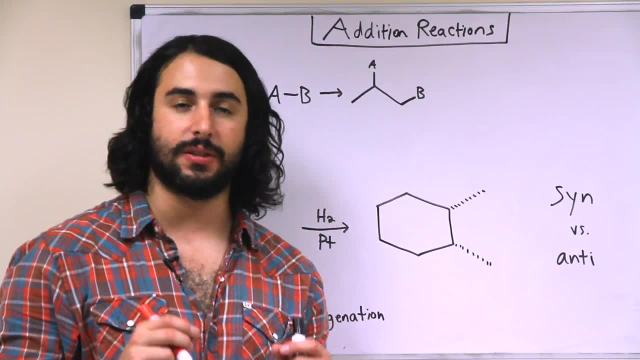 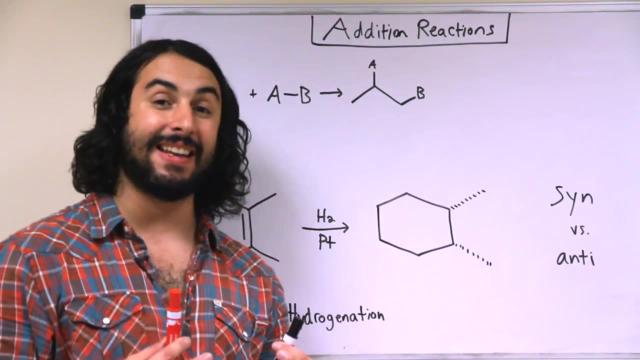 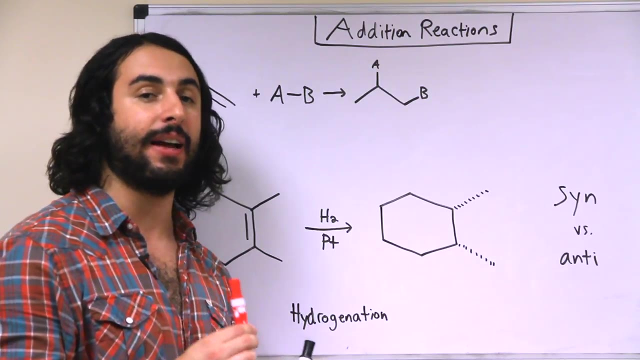 and anti. so those are terms that discuss the stereo specificity of a particular addition reaction. in this case, hydrogenation over platinum metal is a syn addition because the two groups that are being added to the substrate are being added from the same side. so if we take two hydrogen atoms and those are 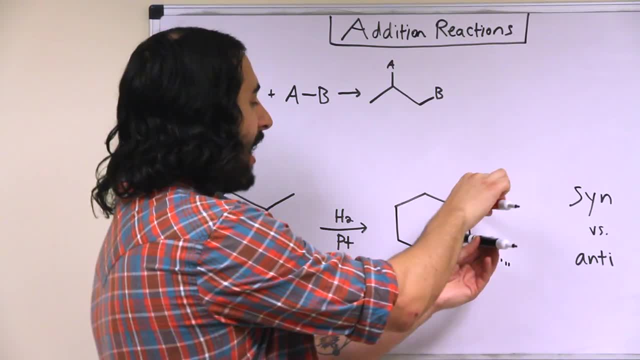 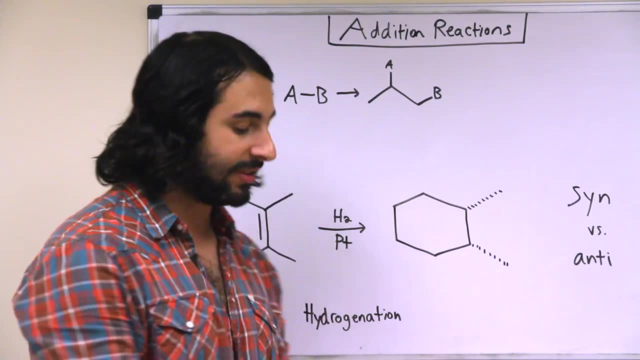 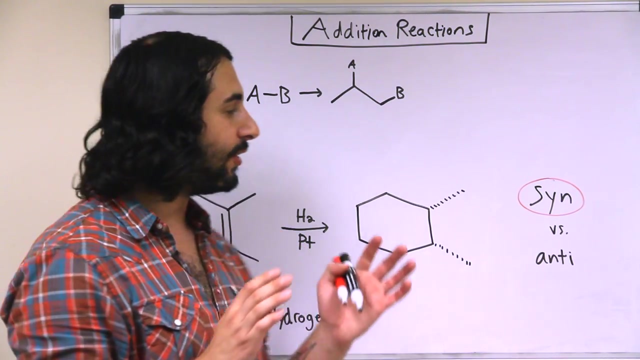 added to the two carbons like that. now the implied hydrogen that were added are on implied wedge bonds, the methyl groups and up dashes, and so this was a syn addition. now it's very important to make the distinction between syn and anti versus cis and 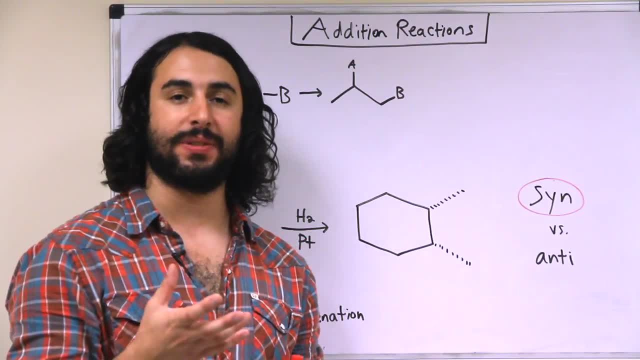 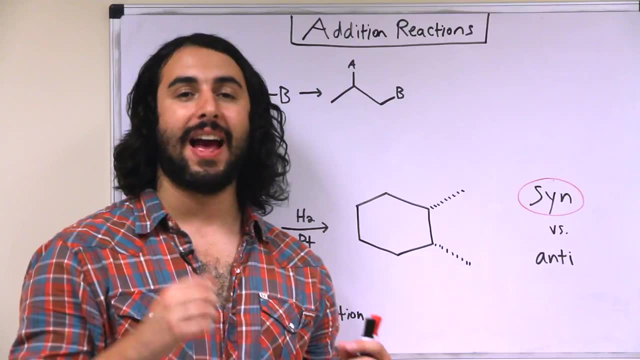 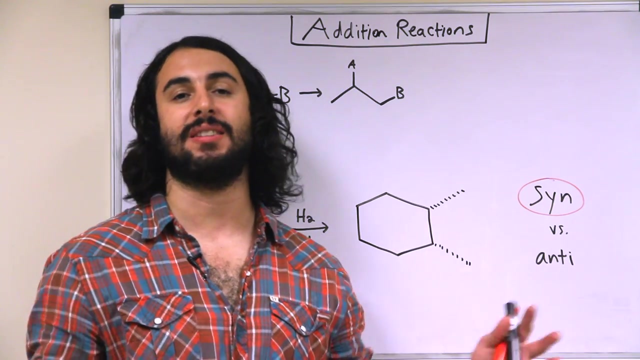 trans. it is true that when two groups are added to a substrate in syn fashion, that they will typically end up cis to one another in the product. however, cis and trans are discussing spatial relations between groups on a molecule, independent of the context of any kind of reaction. 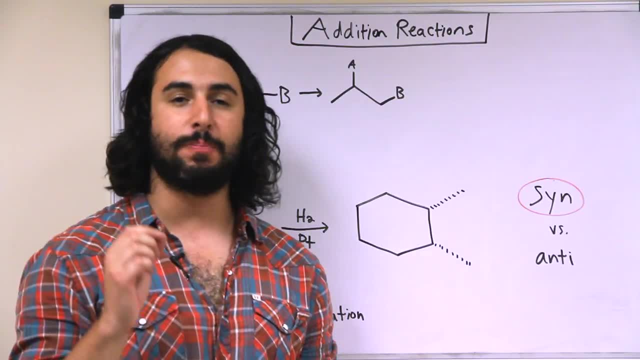 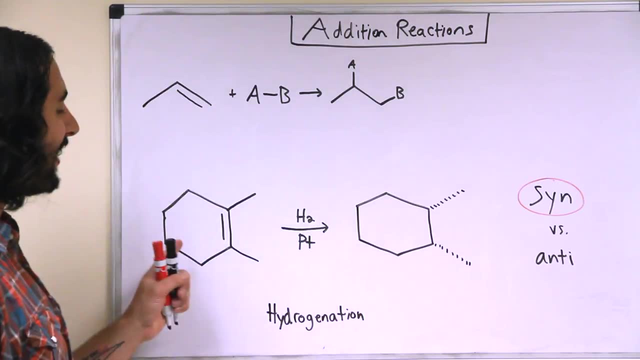 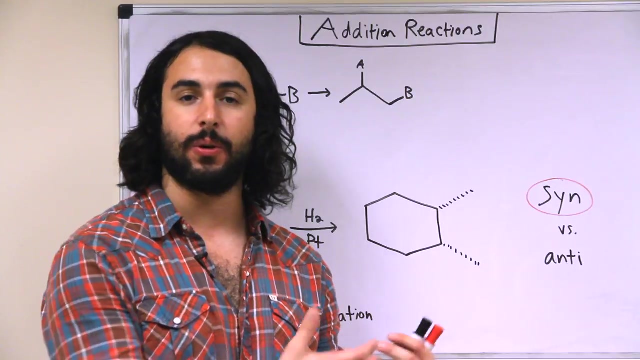 whereas syn and anti are terms that are specifically describing the mechanism of operation of a reaction. so it's within the context of a reaction. this is a syn addition reaction. therefore the hydrogen's that were added will end up cis to one another in the product. so addition reaction: two hydrogen atoms. 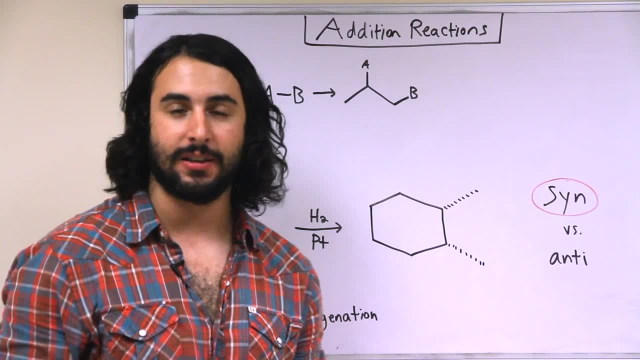 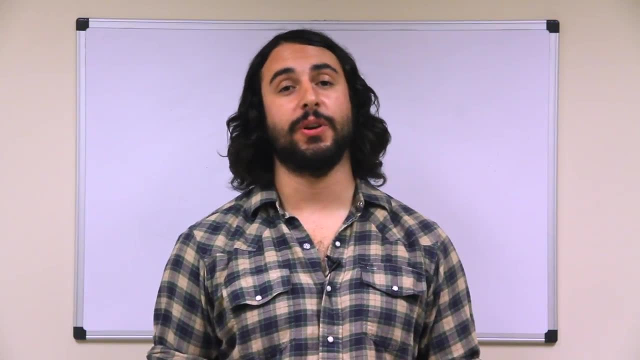 added syn. there they are, in the product, they're implied and that's what we have. thanks for watching. guys subscribe to my channel for more tutorials and, as always, feel free to email me of questions professordaveexplains at gmailcom. 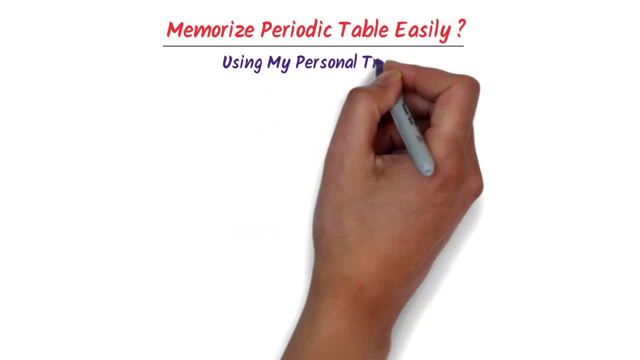 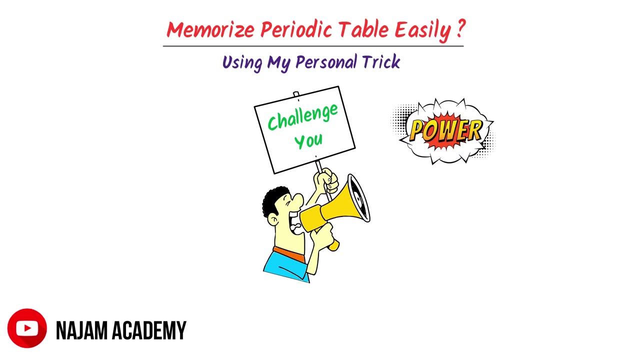 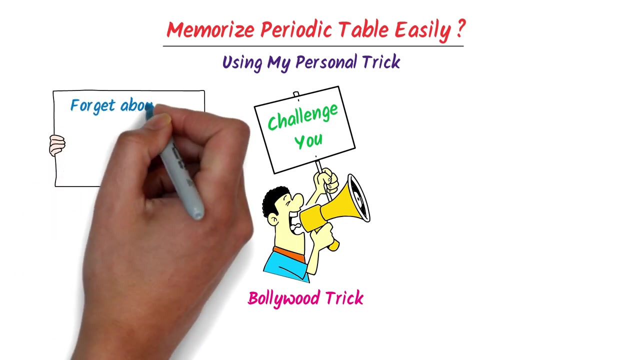 How to memorize periodic table easily using my personal trick of Bollywood pictures. I challenge you that you will not find this trick anywhere, because it is my personal trick, which I called Bollywood trick. Before teaching you the trick, remember that you have to forget about the English grammar. Secondly, if you want to learn the periodic table for lifetime, 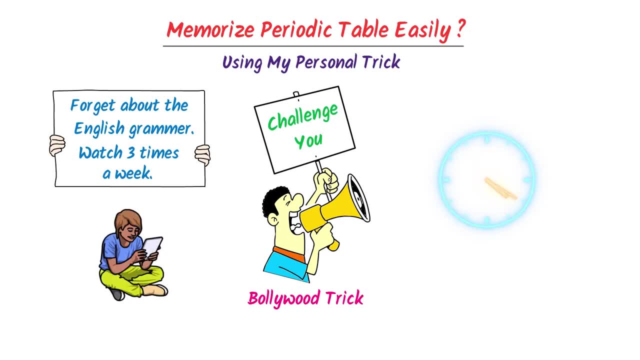 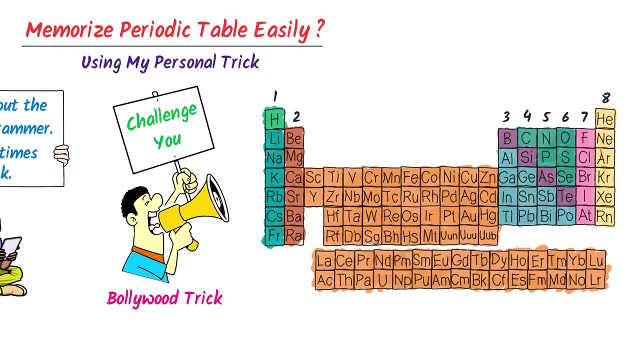 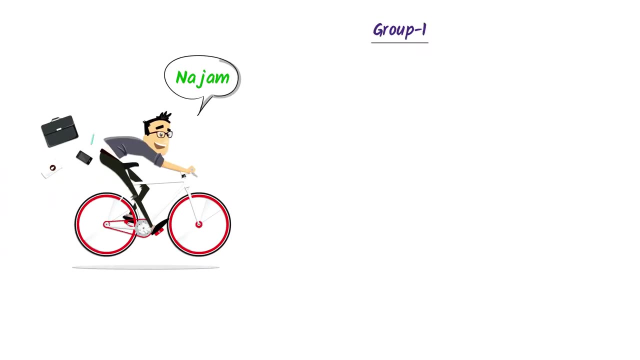 then watch this lecture 2 or 3 times a day for a week. Thirdly, we will learn about 8 main groups and then, at the last, we will learn about transition elements. Now consider Mr Najm cycling fast. I say, Hello, Najm knows running cycle fast. 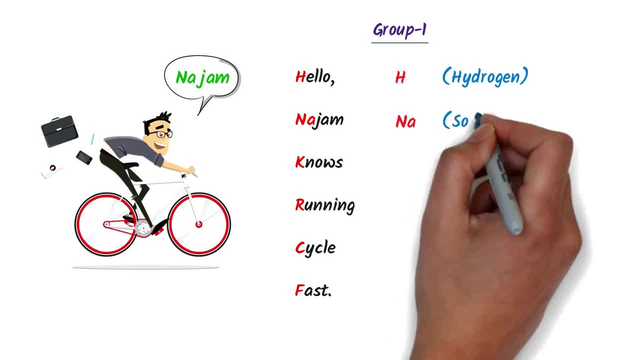 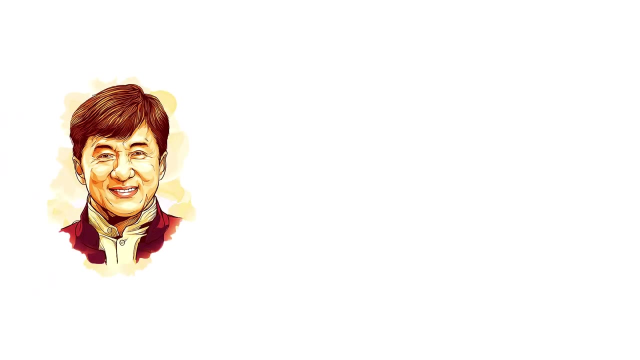 Here: H stands for Hydrogen, Na stands for Sodium, K stands for Potassium, R stands for Rubidium, C stands for Cesium, F stands for Fringsium. Thus, this is the first group of the periodic table. Secondly, consider Mr Jackie Chan. We know that he is very brave man because he can smash anything. 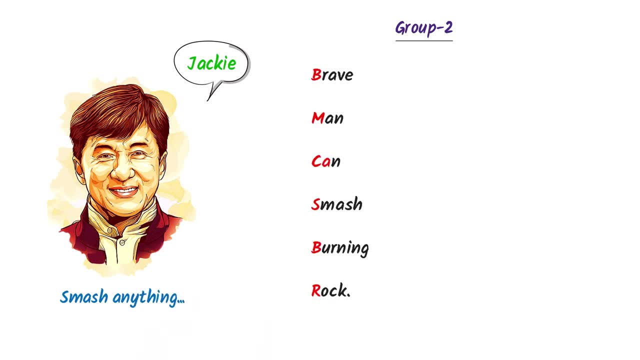 so I say: brave man can smash burning rock Here. B stands for BE, Beryllium, M stands for Mg, Magnesium. C stands for Ca. Calcium S stands for Ca. Coconut ByEM stands forumin tabban. C stands for Celium. the C stands for Al Hyun Se метholam.